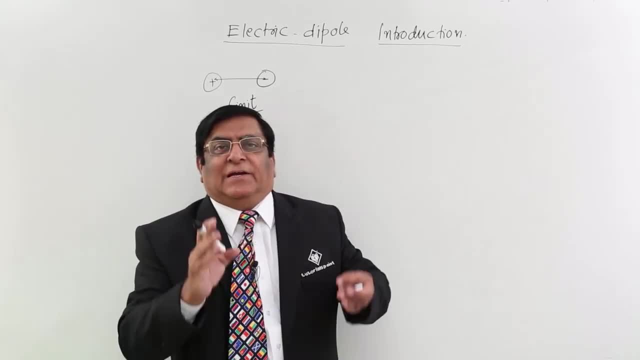 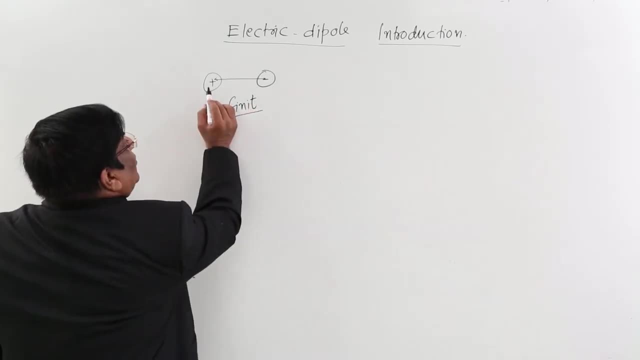 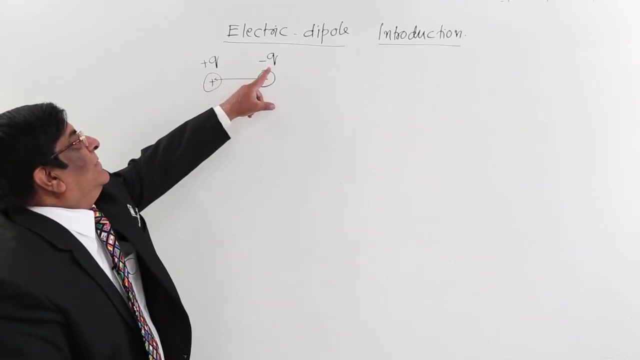 finite, that means it is fixed and it will neither decrease nor it will increase. So there is a finite distance, The quantity of this positive and negative charge. the condition is these two have same magnitude. one should be positive and one should be negative. upright movement 2x. 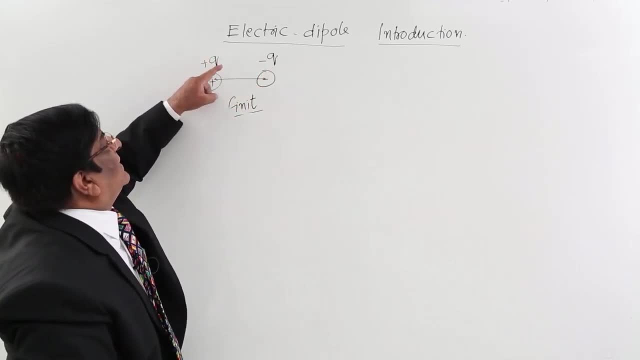 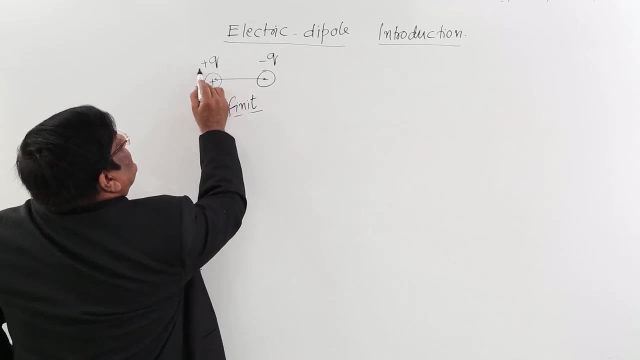 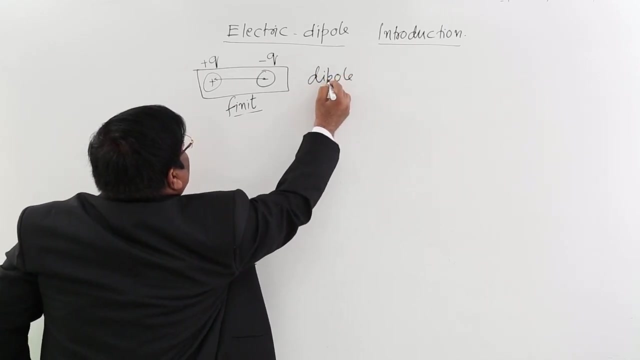 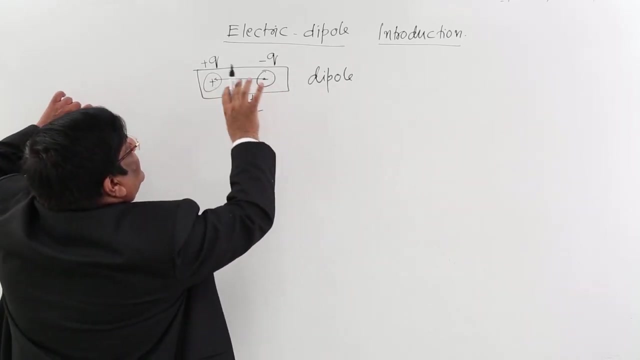 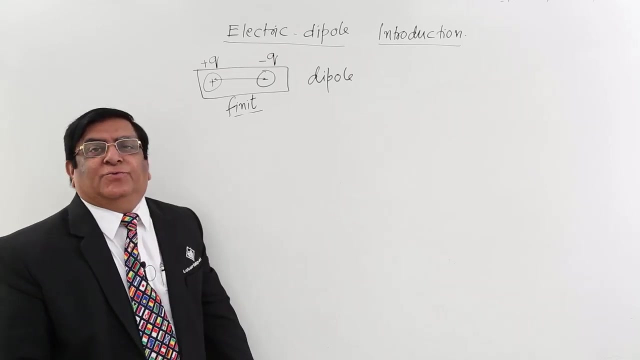 magnitude 25, magnitude 50. magnitude hijo 15 characters, be known as a dipole. Di means two, pole means opposite nature particle. These are two opposite nature particle at the two corners. Therefore this is known as a dipole. ok, Where do we? 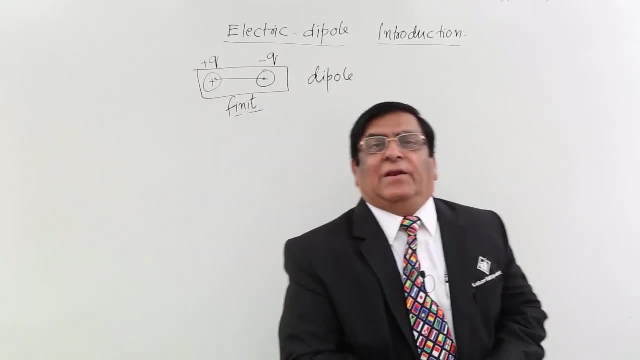 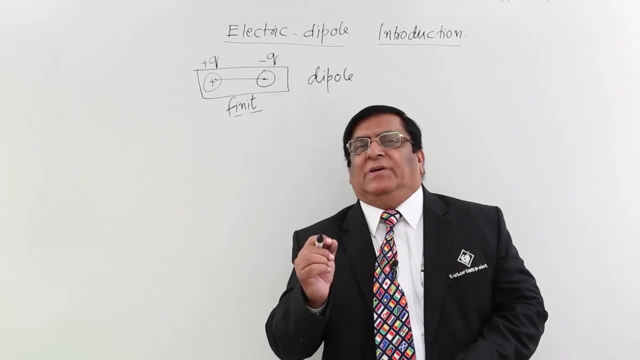 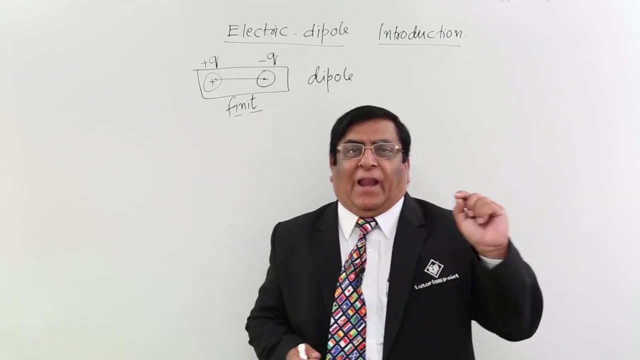 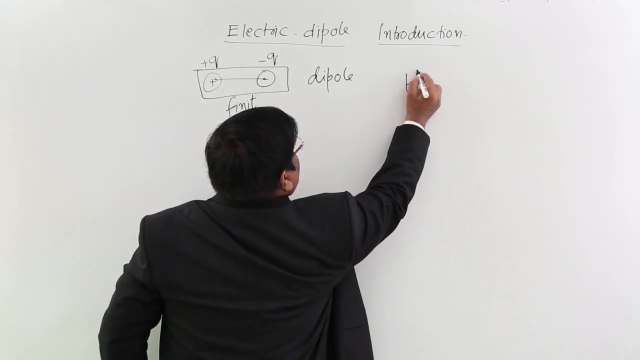 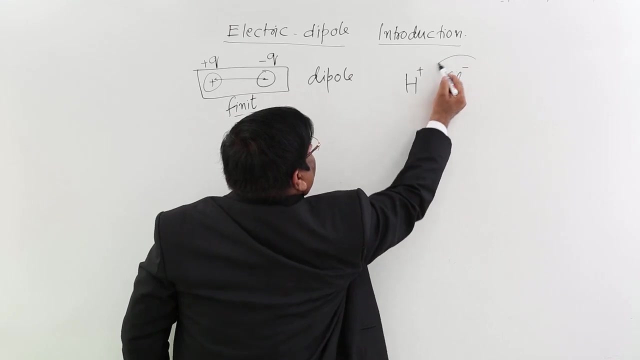 see these dipoles. So answer is: in our compounds, chemical compounds, we have a positive charged particle and we have a negatively charged particle which are bound together, like you know, the acid HCl. HCl, in that H is positive, H is positive and Cl is negative. So HCl. 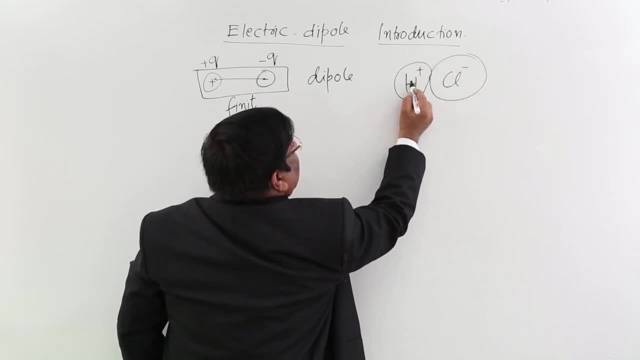 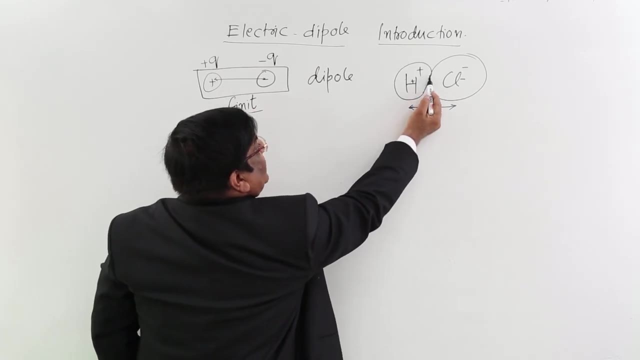 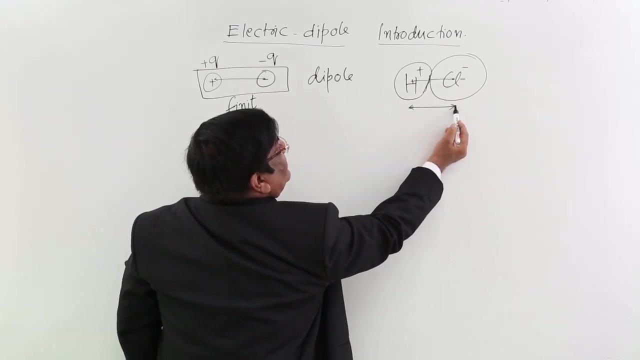 this is Cl, this is H, This is centre of positive, this is centre of negative, And this is the fixed distance, border to border. This is the radius of H, this is radius of Cl and this is the fixed distance between them. There is Coulomb force of attraction. 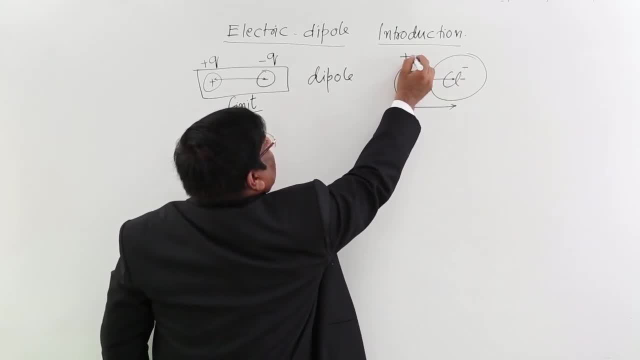 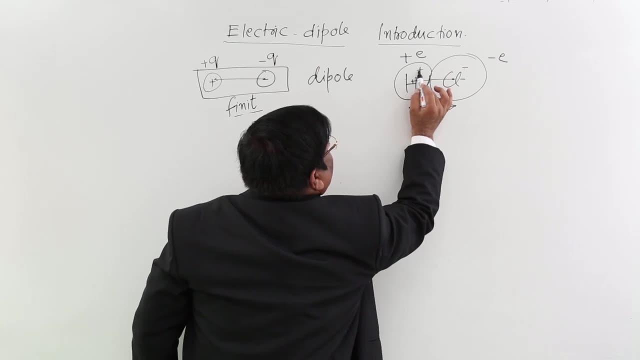 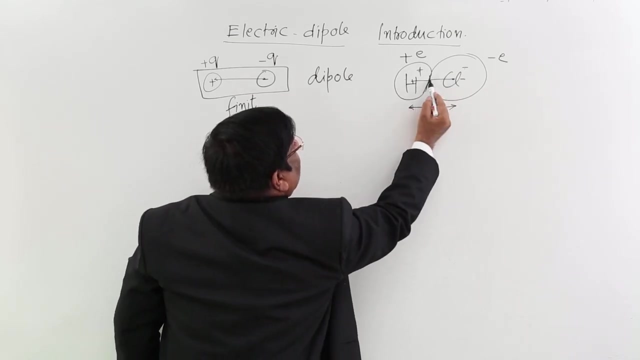 they attract each other. This has got charge plus E. this has got charge minus E because it has lost. it has lost one electron plus E. it has gained one electron minus E, So there is a force between the two and they just stick to each other. So this becomes: 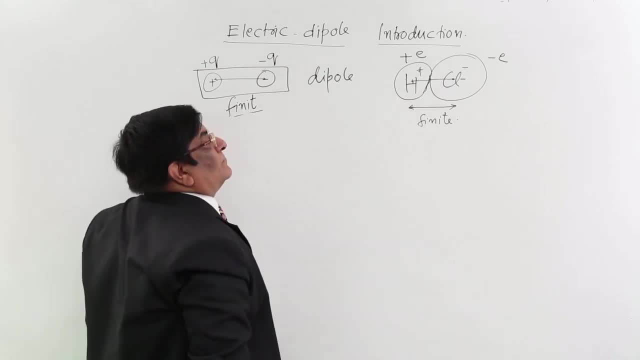 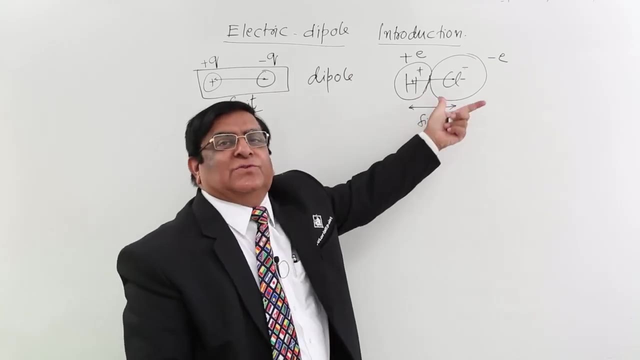 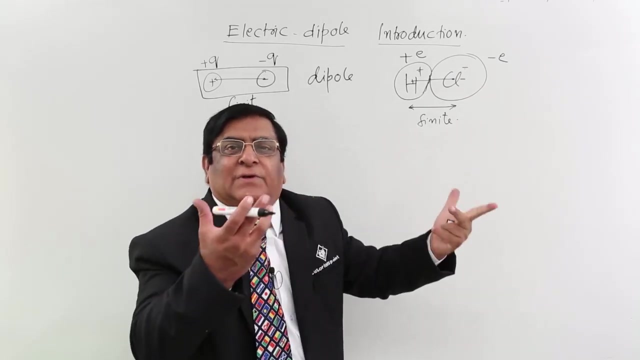 a definite or infinite distance. so equal and opposite charges at infinite distance makes a dipole. So this is a dipole. NaCl is a dipole. H2SO4, SO4 minus, H2 plus is a dipole. So that is why the study of dipole is important. If you are interested, remain in our zrobiće.